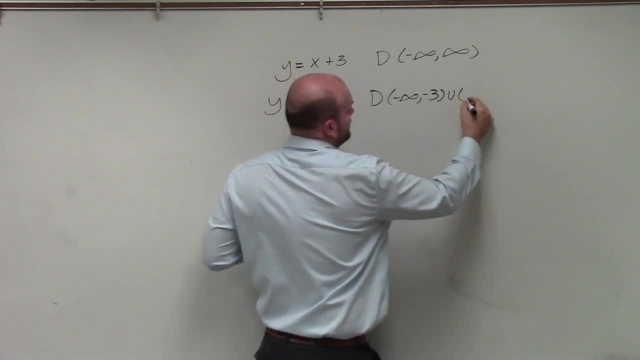 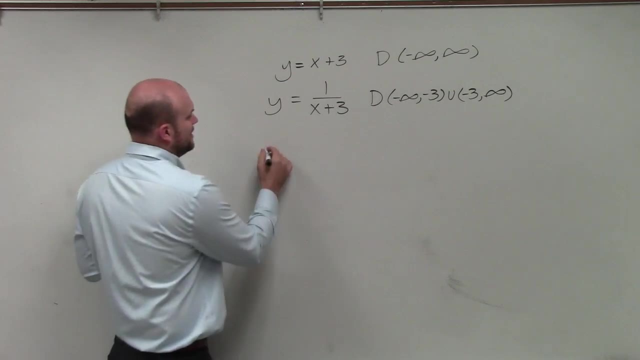 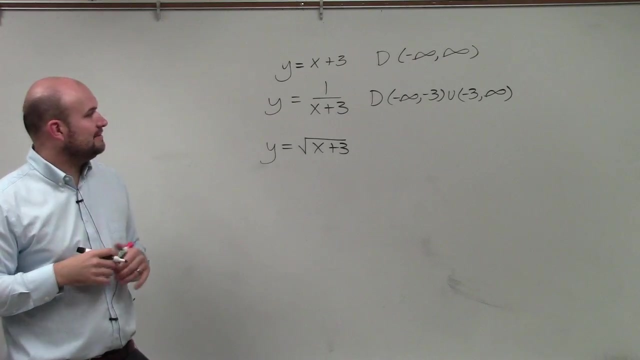 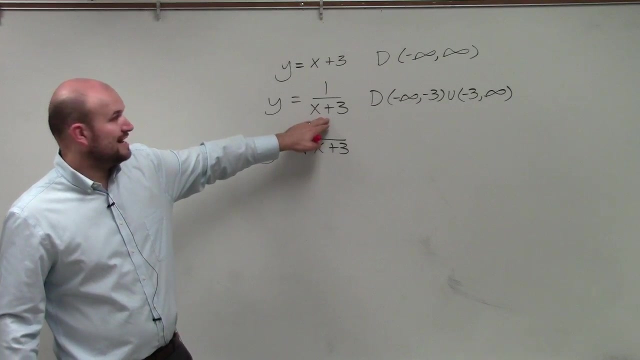 Negative infinity to negative 3. union negative 3 to infinity. Okay, Now let's try the other one. What if I put everything under a radical? Can I divide it by? can I divide a number by 0? in this case, No. However, I understand. oh and again, if you let's say there's a problem where the denominator is more complicated than this, to find what numbers make the denominator equal to 0,. 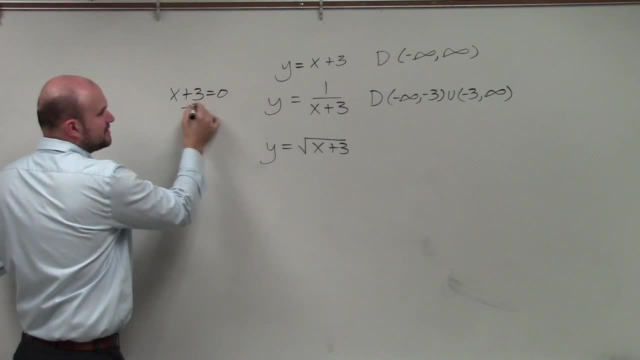 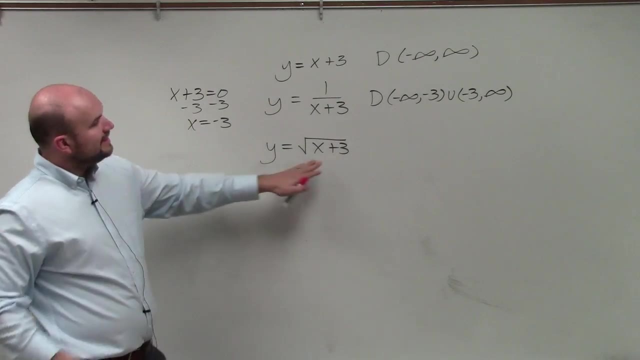 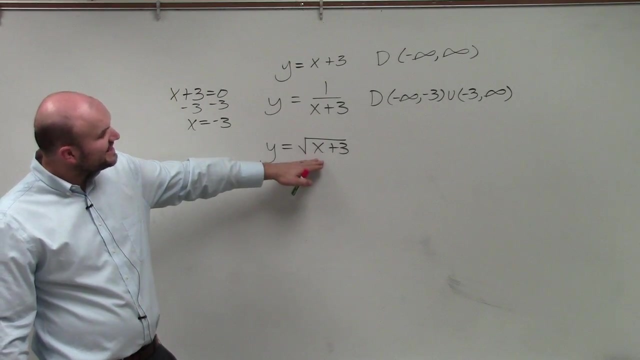 just set that number equal to 0 and solve. That's how we got that negative 3. Just set the denominator equal to 0 and solve. In here, though, we can't divide by 0, so we don't need to worry about this, like this example. However, in this case, you can see that I there's numbers that are going to make my radical negative And I can't divide by a negative number or a negative radical, And you could just think of a number in the top of your head like negative 5.. Negative 5 is not in the domain, Would everybody agree? 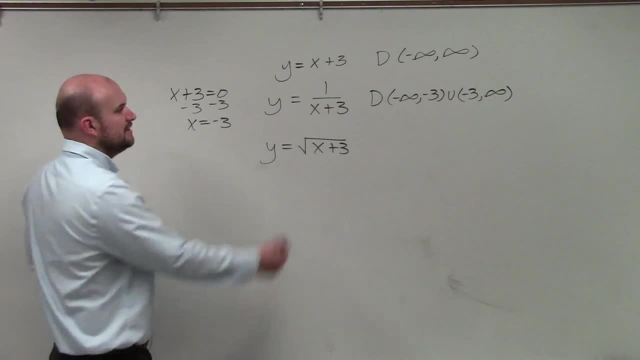 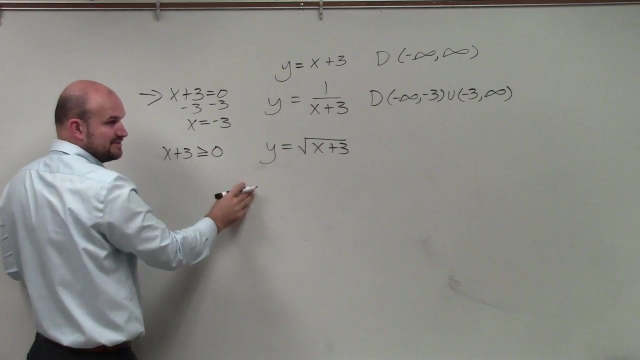 Because that would make my radical, my radical, negative. So how do we determine what numbers, then, are part of our domain and not a part of our domain? Well, when it's rational, we set the denominator equal to 0. When it's a radical, we set our radical greater than or equal to 0. Because it can be 0, you can take the square root of 0. Square root of 0 is just 0. So then we solve: So x has to be greater than or equal to negative 3.. So, going back to algebra 1, we got to say what numbers are greater than or equal to 0.. 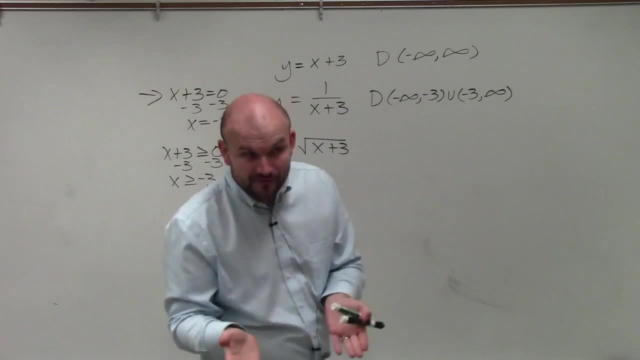 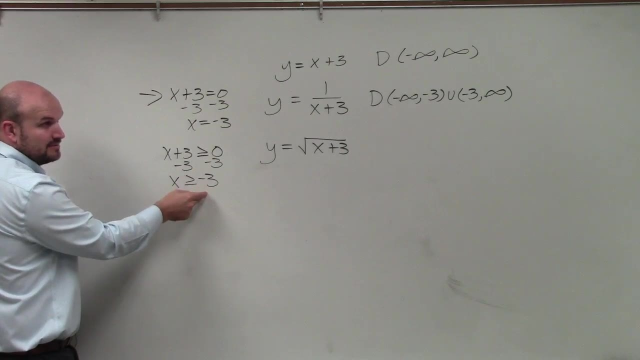 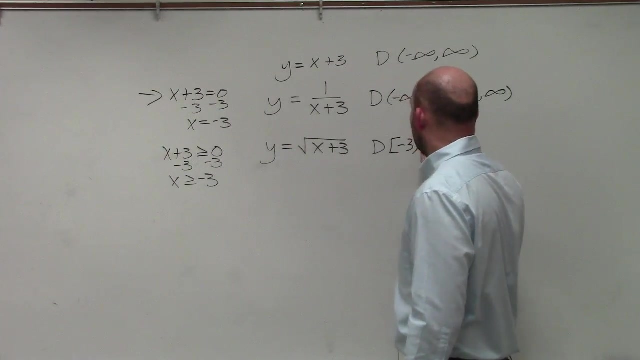 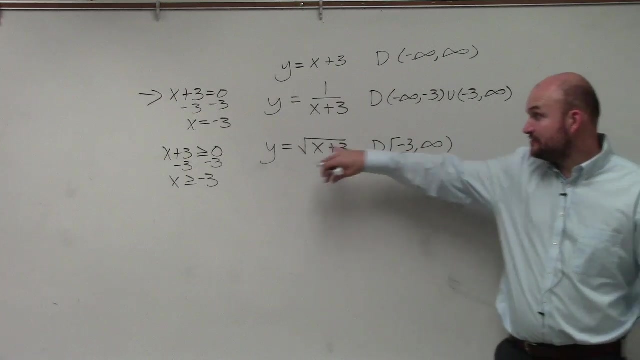 What numbers are greater than or equal to negative 3?? 0 is greater than or equal to negative 3.. Negative 3 is greater than or equal to negative 3.. 1,, 2, all positive numbers, But any number less than negative 3 is not in our domain. So we write our domain as all numbers that are equal to negative 3, but greater than which would go towards infinity. You can be negative 3, because if you plug negative 3, you get 0.. Square root of 0 is 0. That's fine, It's in the domain, But if you do a number less than negative 3,. 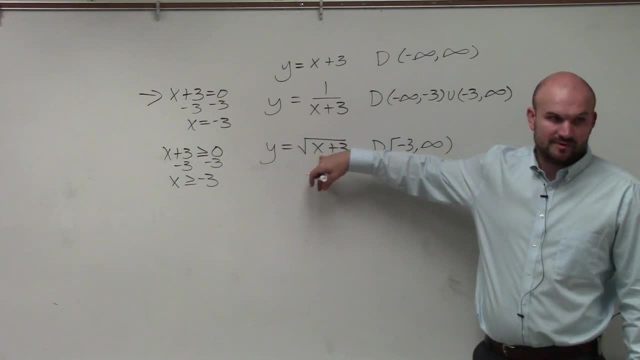 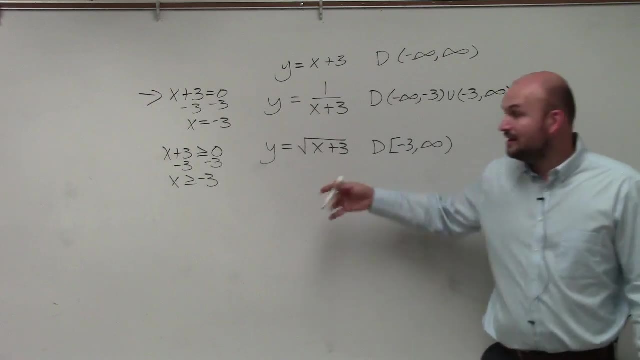 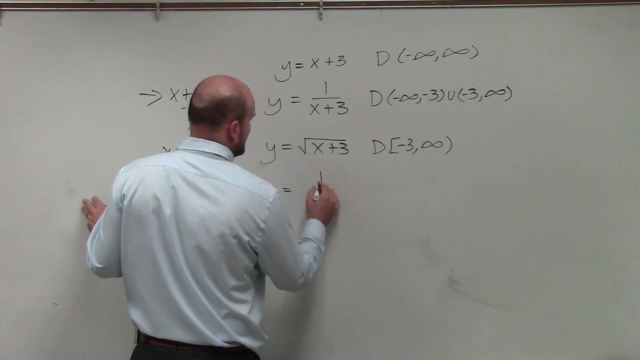 say negative 4. Negative 4 plus 3 is negative 1. We can't take the square root of negative 1 under our real number system. Am I good on my third equation? Then all I got to do is let's just change it one more time.